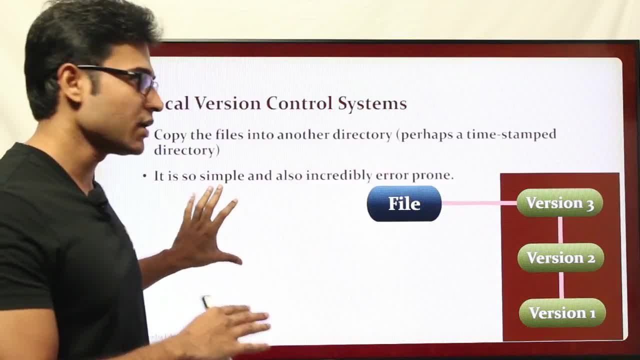 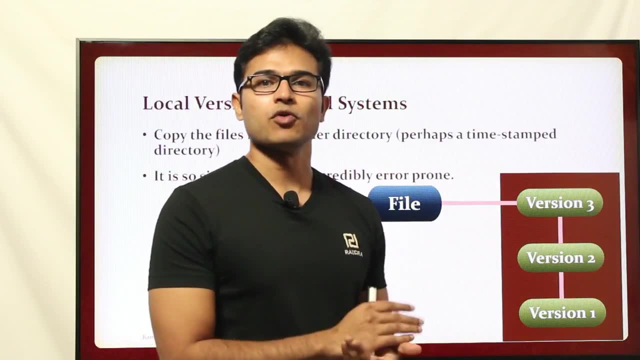 and the other person is going to have all the versions of the code on his own computer and whatever changes both of them are making, they will not be reflected or both of them will not know about it. So the option is have a central database which is going to maintain all these versions. 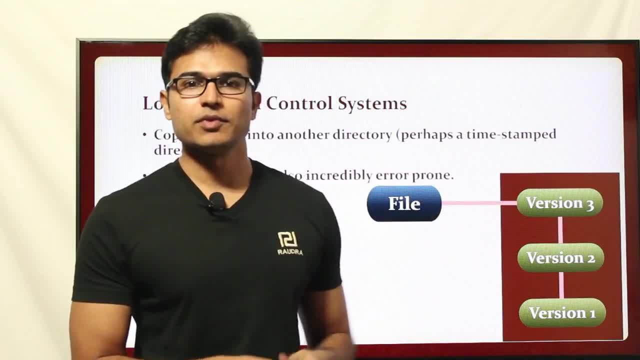 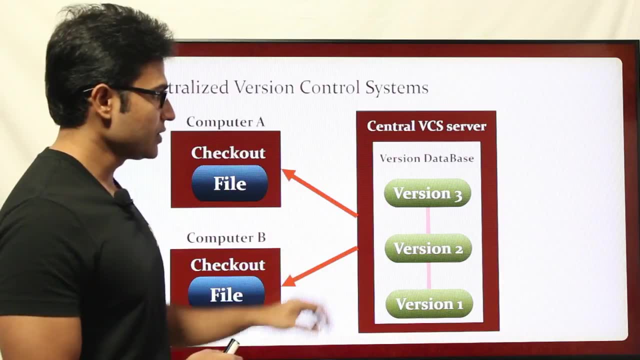 so that if someone makes the changes, other person should be able to see it. Let's see that model Now. if you observe here, now in the evolution, the next step is when people are working on the same project, then they will come up with a central VCS server. 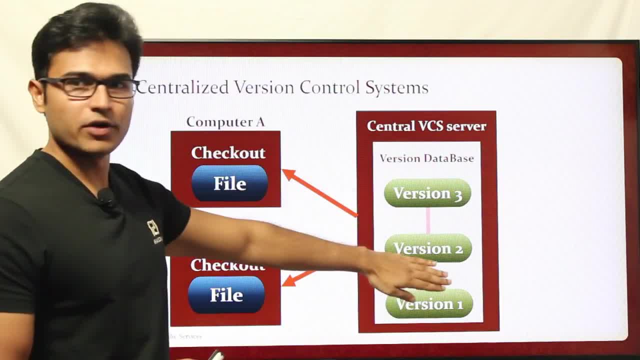 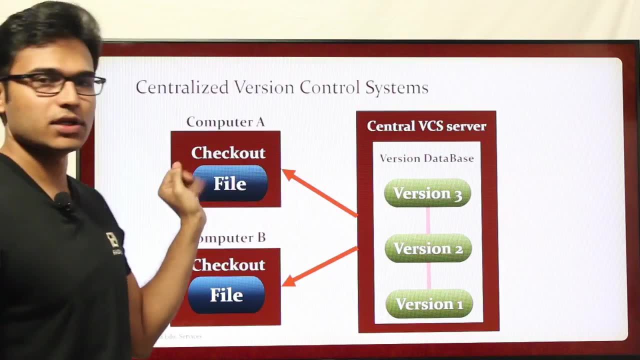 In the central VCS server. they are going to maintain all the versions and now whoever is working on it, they can get whichever version they want and then they can check it out. So see this Now. let us say on a computer, A one person is working on the same code. 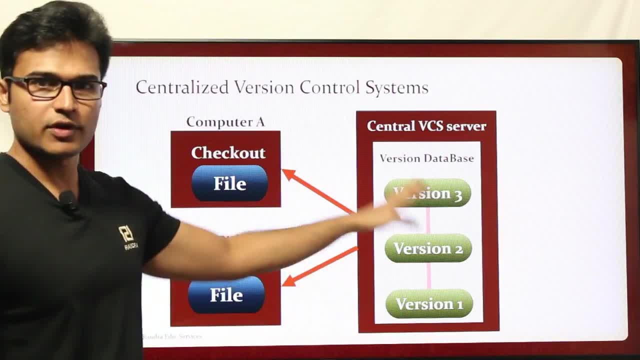 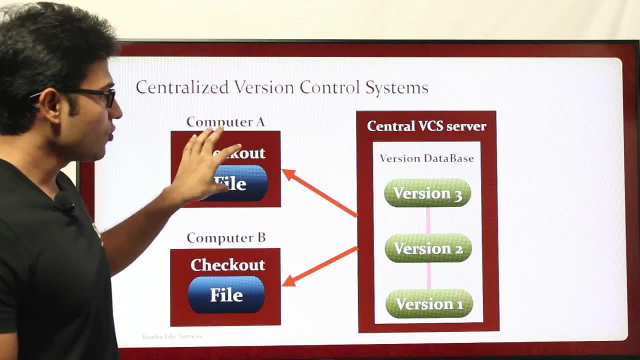 and the computer B. some other person is working on the same project. Both of them are working on the same project. Now they can get whichever version they want and then they can make changes. But then the problem in this model is both of them are seeing the central database. 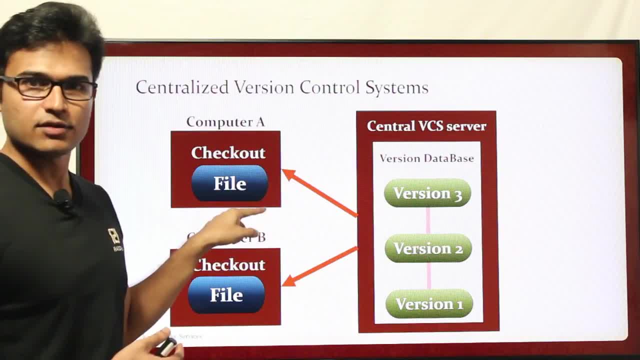 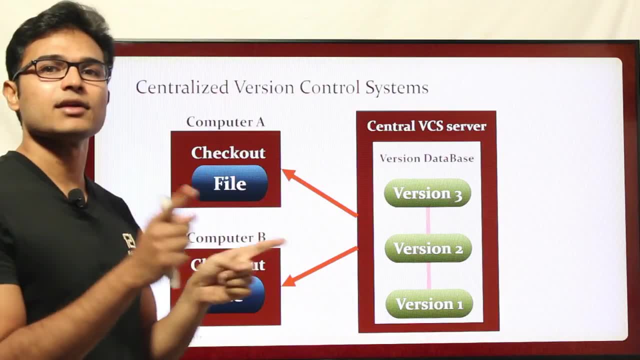 but then both of them are not communicating with each other, Which means if some person makes the changes and other person also makes some changes to the same line, assume that both of them are making the changes to the same line- then which change will be updated to the database? 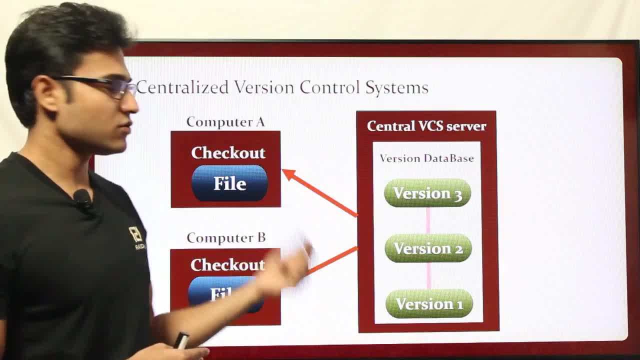 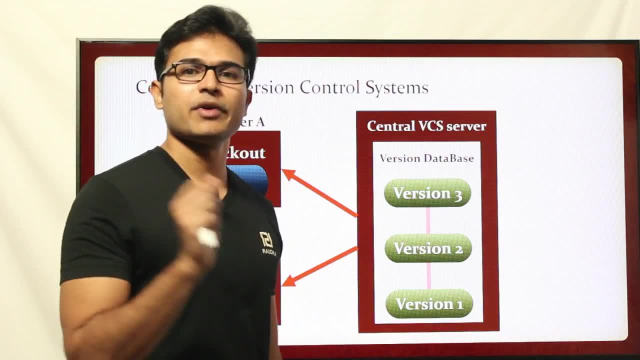 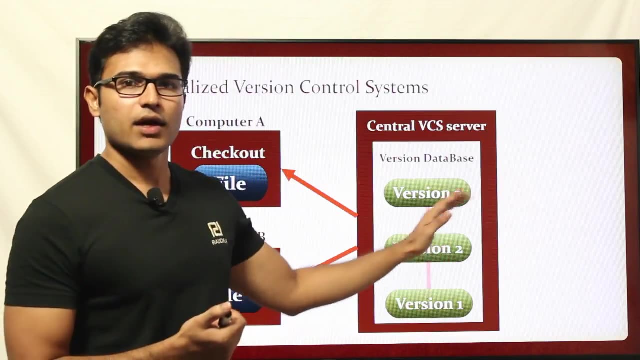 That depends on who updates it last. So because of which there is a chance that, if you remember, or if you have any knowledge about operating systems, there is something called as race condition. Race condition means whoever updates the code the last, their changes is going to be there. 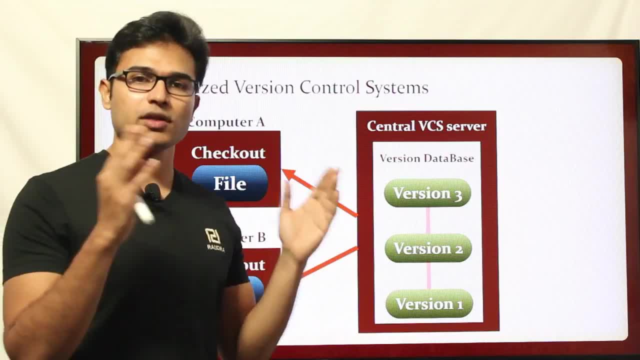 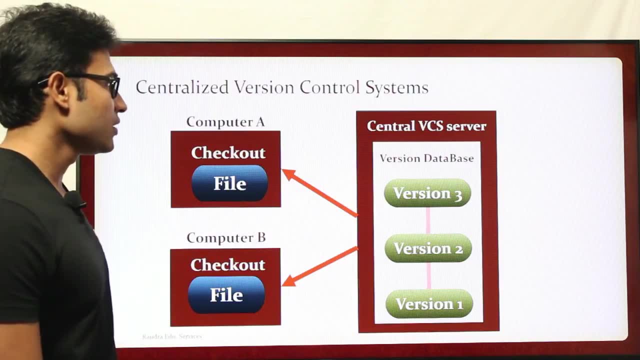 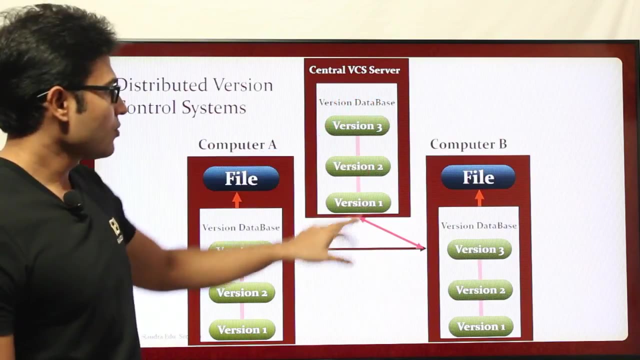 and the other changes will be discarded, And you don't want that to happen. Then even these two computers also have to communicate. So that is the next model in the evolution. Now, if you look at the next model in evolution, this is the central database, and both these computers are communicating with the central database.